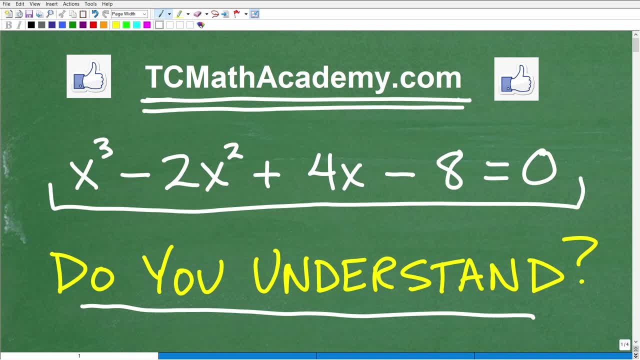 You can find a link to that in the description below, And if this video helps you out, don't forget to like and subscribe, as that definitely helps me out. Okay, so let's go ahead and take a look at the answers right now. 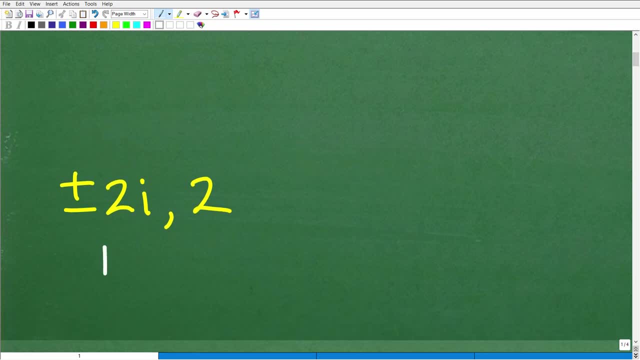 So here are the solutions to this equation. So we have plus or minus 2i and 2.. So here we have a complex imaginary number as two solutions. And then we have a complex imaginary number as two solutions And of course we have two is a real number. 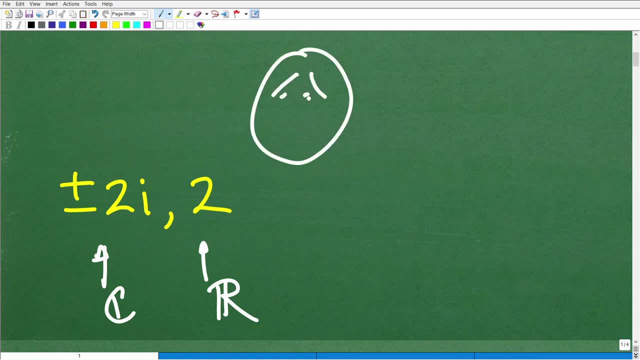 Now if some of you out there are looking at this and be like, oh my goodness, Mr YouTube math man, I'm totally lost. I desperately need help in this. Well, don't panic, I want to explain to you, kind of you know obviously- how to do this problem. 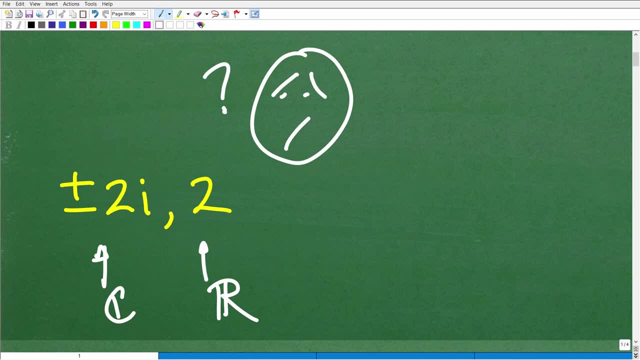 And I'll give you some suggestions on how you can learn this. But, again, you may not have taken this yet And, anyways, I'll give you more information on what exactly what I'm talking about in terms of the level of math that we're dealing with. 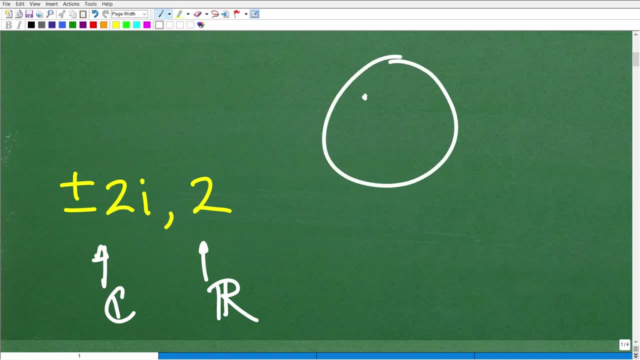 But if you guys are interested in this, if you got this all right, that is very impressive. Matter of fact, you definitely earned a happy face and a plus a 100 percent and a few stars, So you can tell your friends and family that you know exactly how to solve a drum roll. 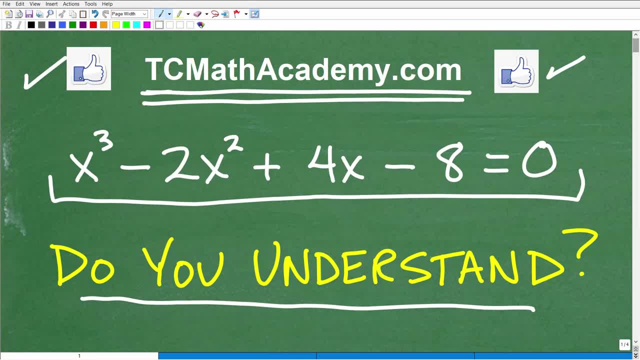 I'll tell you what this is. We are talking about a third degree polynomial equation. OK, so the directions here would be: find the roots of this polynomial equations, ie solve this polynomial equation. So, anyways, I'll give you some suggestions on how to solve this polynomial equation. 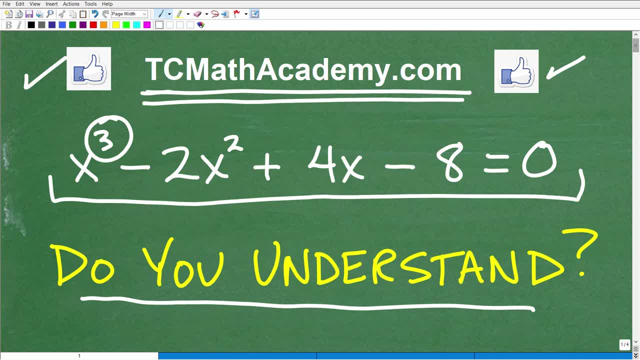 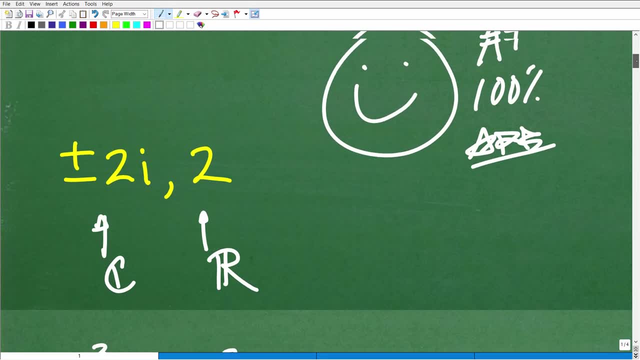 I'll get into this right now in terms of fully explaining what's going on, But if you understood this, that's a very, very good. Clearly you are paying attention into in your class, or maybe you've been watching a lot of my videos. 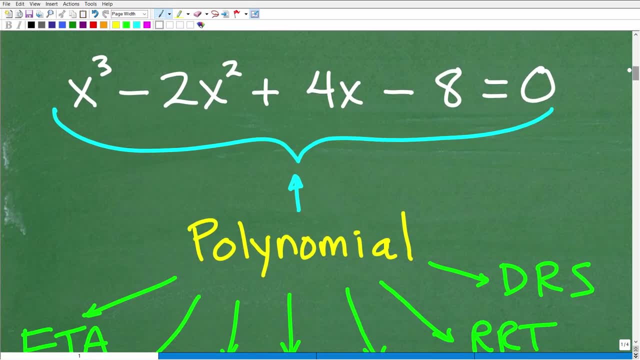 Who knows? Let's get into the problem right now. OK, so here is the polynomial equation in question, And the first thing we need to recognize is we're trying to find the roots to this. Now, of course, I'm telling you: it's a polynomial. 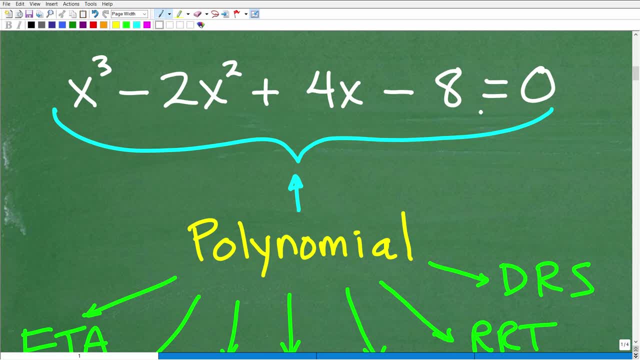 Suppose I said, just solve this thing, All right, And you're like, OK, no problem, I'll solve this thing. You would have to first determine what are you dealing with. OK, there's a different type of equations in algebra and they're not all polynomial equations. 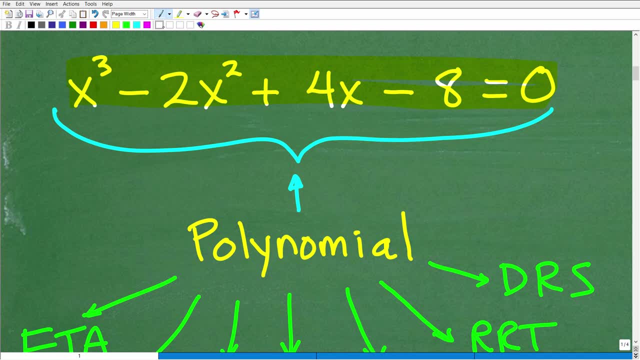 You can have logarithmic exponential systems of equations. you know quadratic. Well, quadratic equations are actually polynomial equations, But there's all different sort of radical equations, on and on and on. So not every single thing, Of course, is going to be a polynomial. 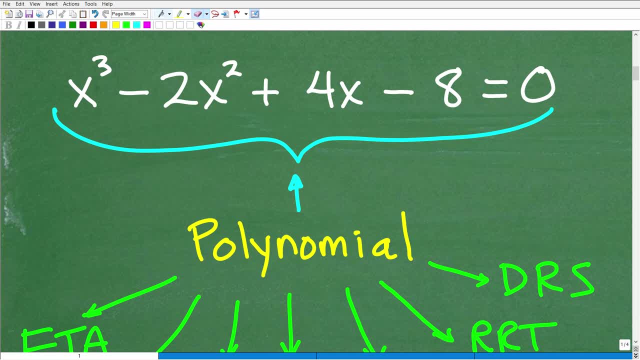 So you have to be able to recognize that In fact, we are dealing with a polynomial. OK, now, a polynomial will have terms and we have your variables right here. And this is just a real quick, loose definition of a polynomial. 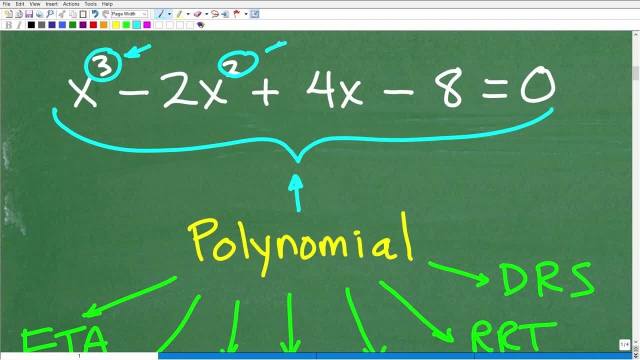 Basically, you're looking at the exponents, of the exponents on the variable terms. OK, you can't have any negative or decimals. Basically, you're looking at positive whole numbers. All right, You could have Well zero, Yes, that's the positive. 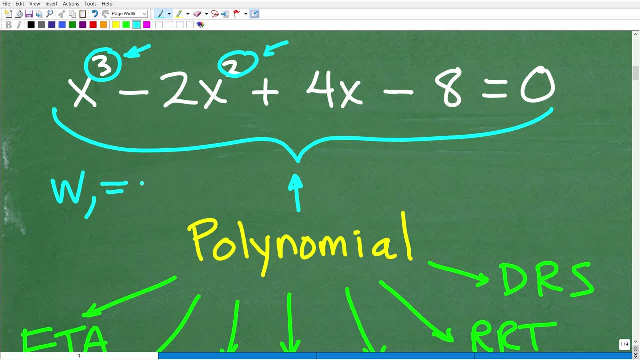 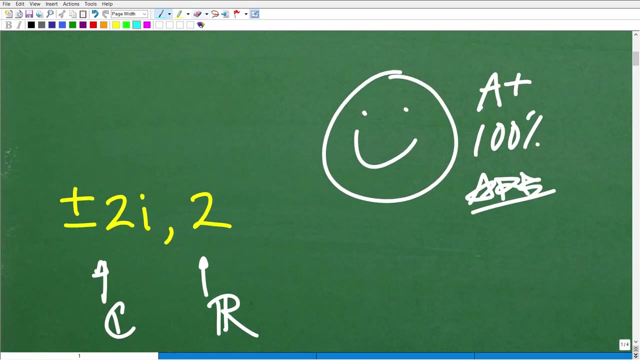 Well, that's the whole numbers, OK, which is includes, or includes, excuse me, zero, one, two, three, on and on and on. These are the only things that are allowed on in terms of your exponents Right. So, for example, let's suppose you had something like this: 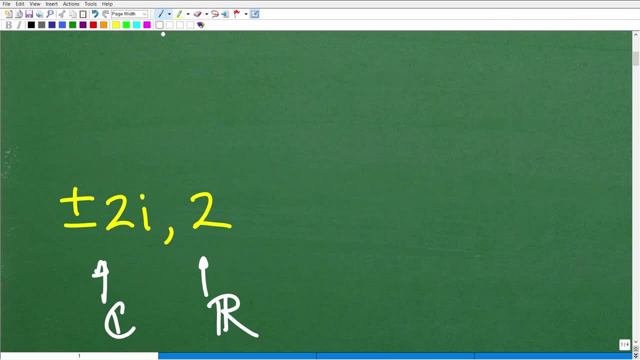 And this is important because you need to understand- one that you're dealing with a polynomial. So if I have X to the two fifths plus X, So if I have X squared minus three equals zero, this is not a polynomial, not, not. not because this exponent up here is not a positive whole numbers on an integer or positive integer. 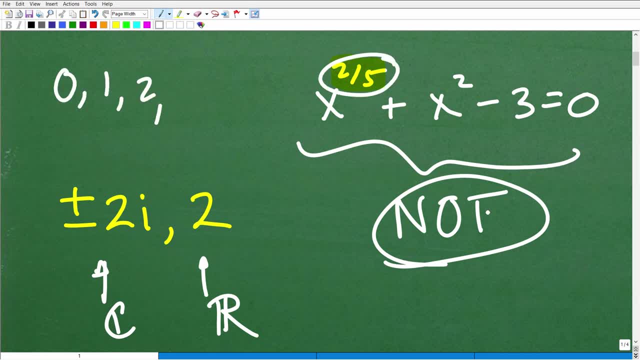 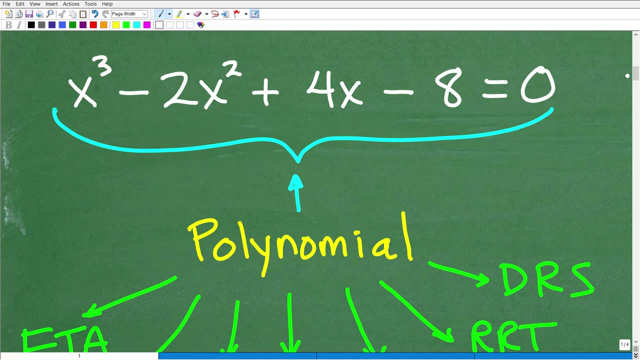 Right, It's not zero, It's not one, It's not to. you got this situation. So this is not a polynomial, which means you'd have to use other techniques, But we love polynomials in mathematics and even more advanced mathematics like calculus. 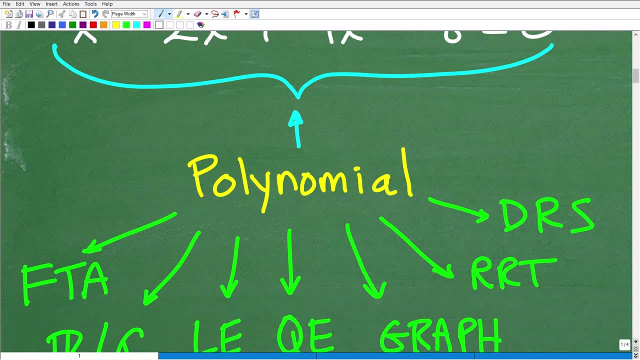 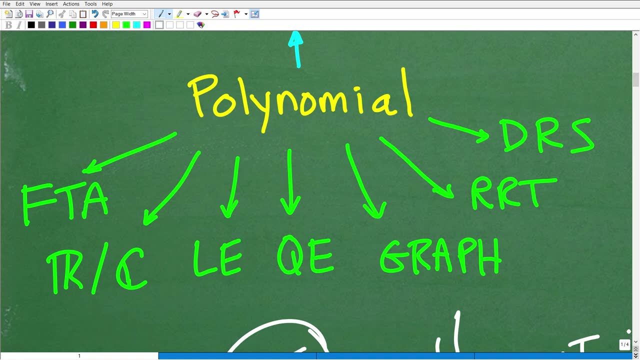 So polynomials is a huge topic that you study in algebra, pre-algebra, algebra one, algebra two just continues on. So first things first. First, we need to identify: Yes, indeed, it is a polynomial. All right, So you can see at all this crazy stuff written out here. 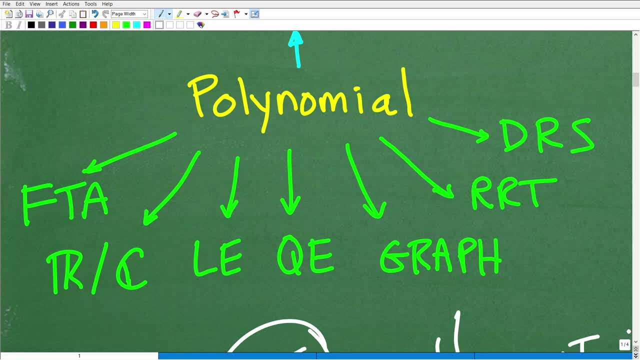 Let's just talk about some of the things that you need to know about solving polynomials, polynomial equations. So the first thing is the fundamental theorem of algebra. So what does that mean? Well, let's go back up here real quick, And of course, this is not. 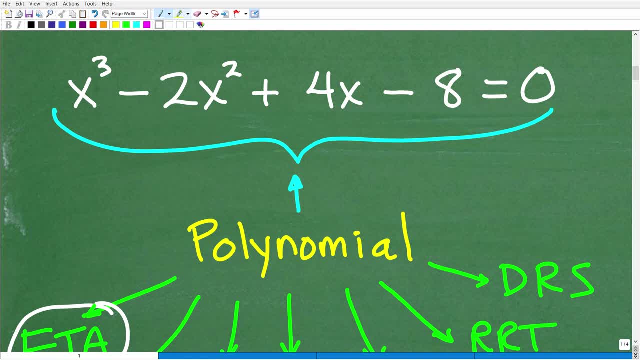 Like a full lesson on this, but effectively what the fundamental theorem algebra basically states is that whatever the degree the highest power of your polynomial is, that's how many solutions you will have. So this third degree polynomial is going to have three solutions. 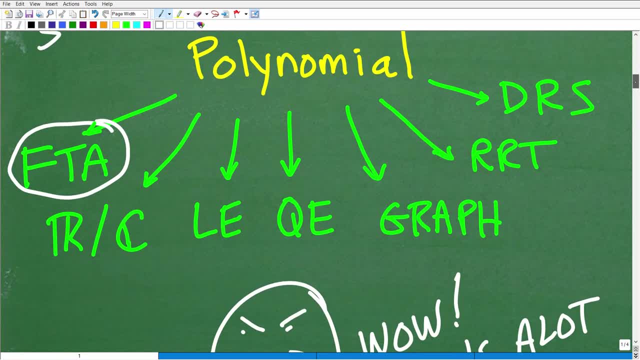 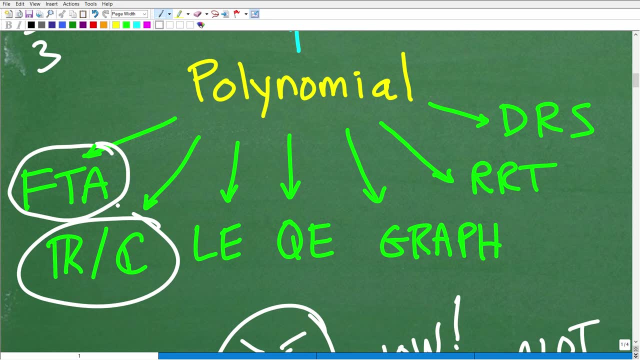 Now what type of solutions you can have: real and or complex type of solutions. that brings us to our next thing. So you just don't know. You can have a real number, Or imagine Or complex numbers. In this case we see if we have one real and two complex and imaginary numbers. 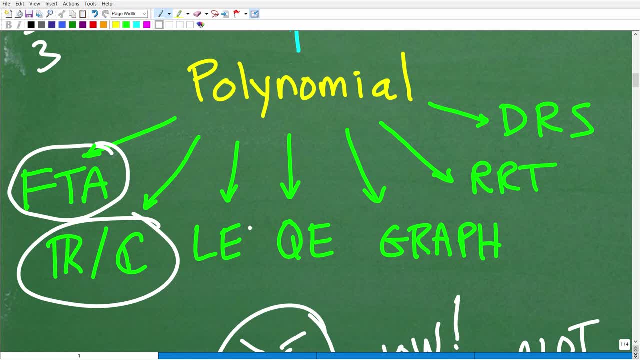 Now other things that you know already, should know about polynomial equations is just solving basic linear equations. I'm talking things like two X minus three equals seven. This, of course, is not a linear equation, but it is a basic polynomial equation. 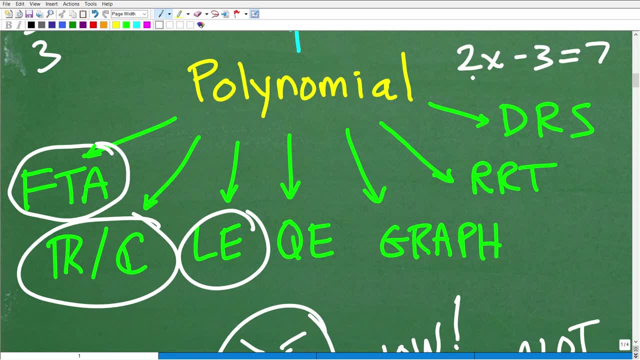 It's a one degree polynomial equation or polynomial equation, Excuse me. And then, later on, and like your first year algebra, you start learning about quadratic equations And all the techniques to solve quadratic equations, to include the quadratic formula. OK, but again, this is a subset of all the stuff you learn about polynomials. 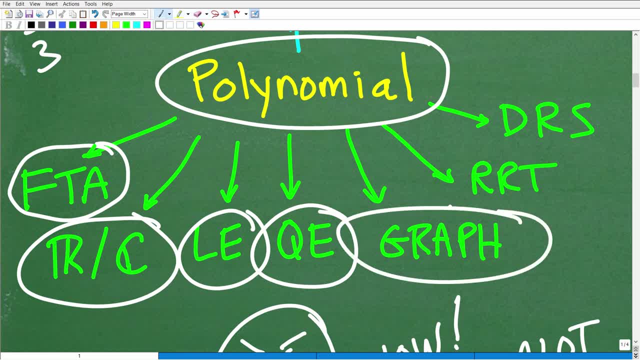 All right, let's continue on. Next thing is graphing. So when you have the graph of a polynomial, you could- you could basically get all kinds of clues, exact to, to see what's going on in terms of the roots. OK, so graphs are awesome and you need to know how to graph polynomials. 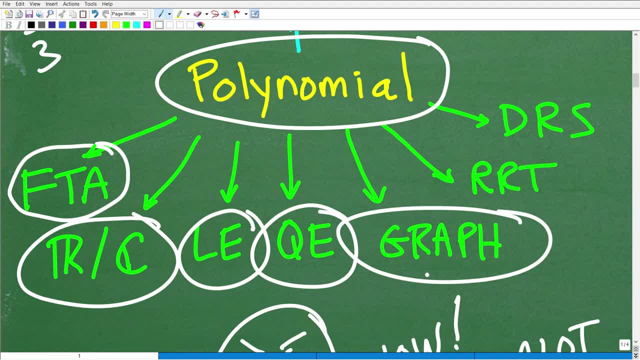 But we're going to review, We're going to refrain from graphing polynomials, We're certainly not going to use our calculator, but you definitely need to know about this And again, it's part of kind of the knowledge that you need to know about a polynomial. 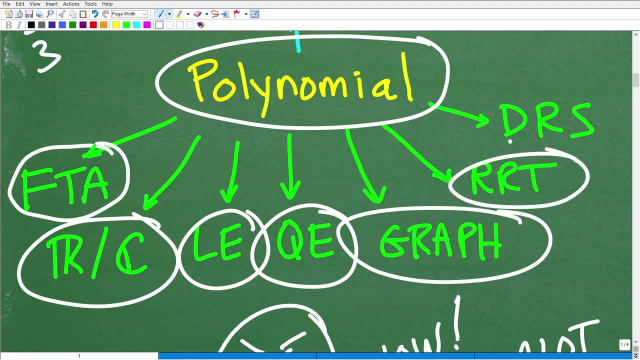 Now here's some other things that are very, very important We have. when you get into like more advanced algebra, which we're dealing with right now, you start learning all sorts of kind of new theorems. OK, one of the one, one of which is the rational root. 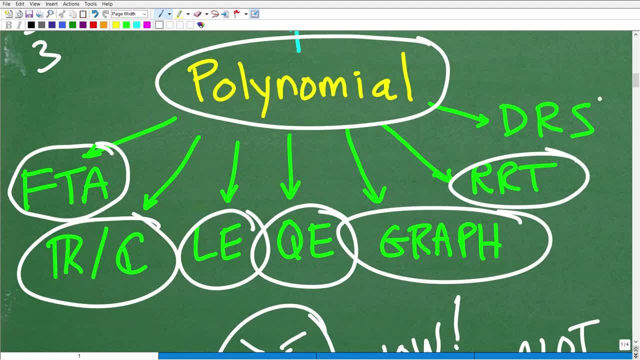 Theorem. There's other ones that you need to know about, And then here you get Descartes rule sign. We're not going to talk about this, We are going to use this, but these are just the tools that we have when we're solving polynomial equations. 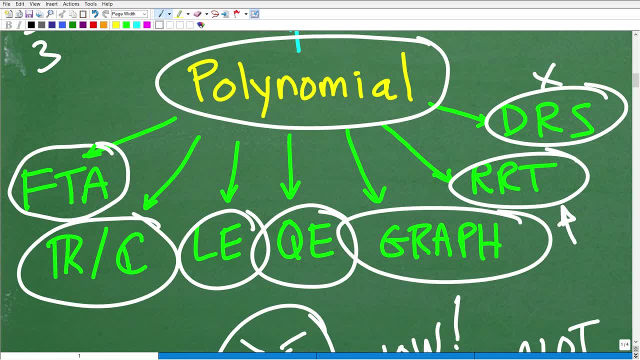 OK, now, if you really want to learn this kind of advanced stuff, I would suggest you either go to my algebra two course, which is effectively the same stuff you're going to get in college- algebra. So that's going to take you one level of kind of advanced mathematics. 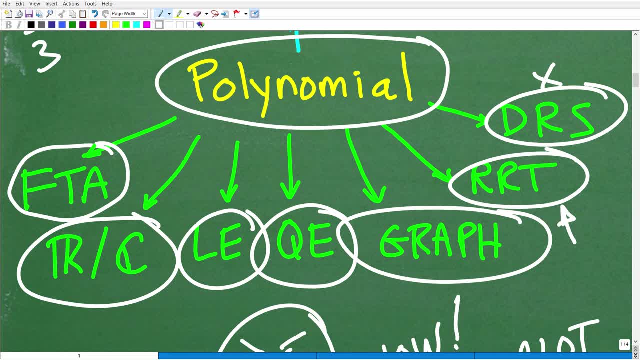 But if you truly want to, To max out in terms of all the stuff you need to know about polynomials, I would strongly encourage you to check out my pre calculus course that I get into Descartes, world signs and all kinds of other good stuff. 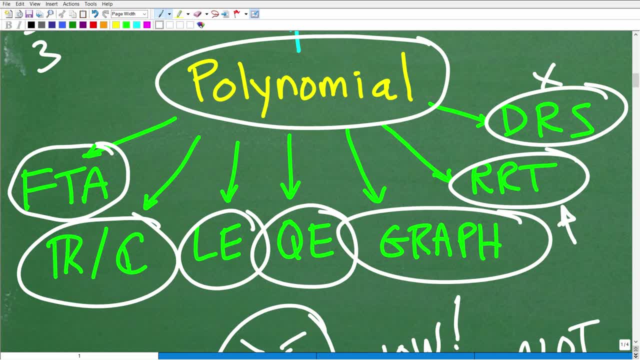 OK. so if you're not familiar with any of this, well then, you know, you likely haven't studied this yet. But if this is like ringing a bell, you're like, oh yeah, I remember rationing with theorem and yeah, I kind of remember something about it. 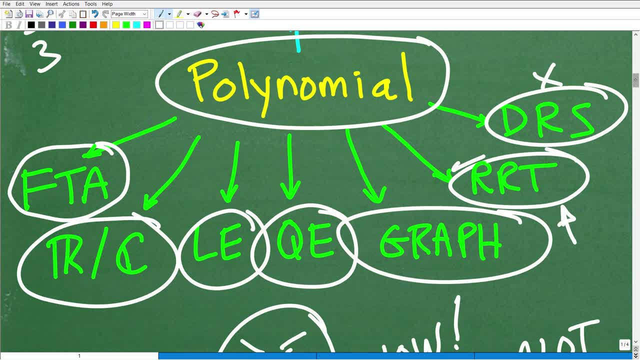 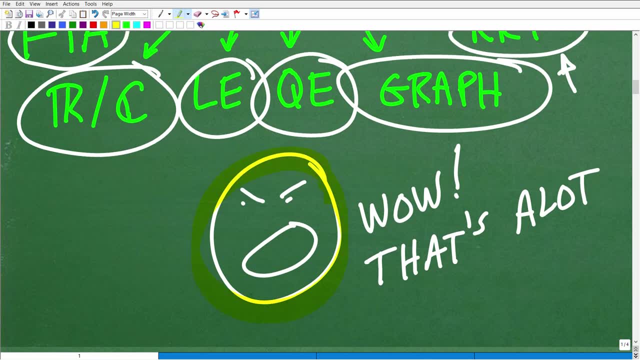 Then that means that, hey, you probably were taught this, But let's go ahead and get into how to do this, How to do this problem. So the first thing is: you know, of course I like to have fun with my little tablet. here is like somebody might be saying, wow, that's a lot of stuff to remember and keep you know in mind. you know, what do I even do? 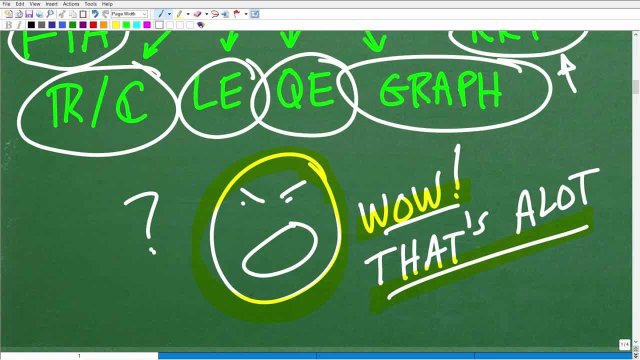 This is so confusing. Well, here's the deal right: Learning something you know like taking notes from a teacher. That's one level of learning, But it means nothing unless you actually do prompts and apply that knowledge And the only way you're going to gain like full comprehension or synthesis. 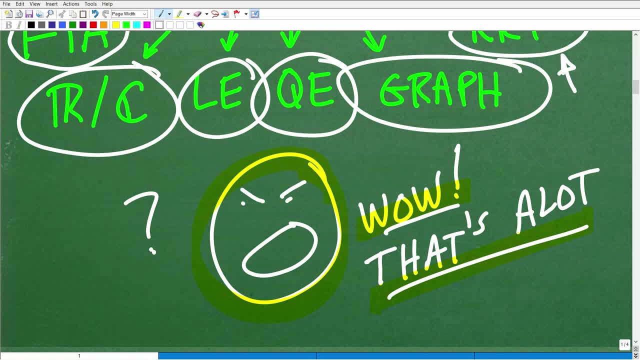 Of all these different concepts is to practice. OK, so it is a lot of information, But again, that's why math, you know, is cumulative and it takes you know years to build up this kind of knowledge. But let's go ahead and get into the problem right now. 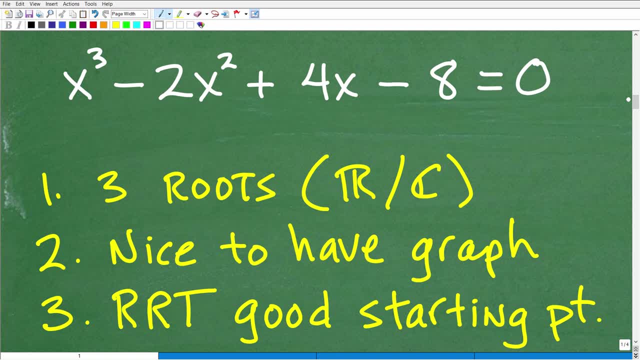 OK, so here is our lovely third degree polynomial equation, And the objective is to find the roots. What are the roots? When you hear this word roots, you might hear another word: zeros, roots and solutions. And you might hear another word: zeros, roots and solutions. 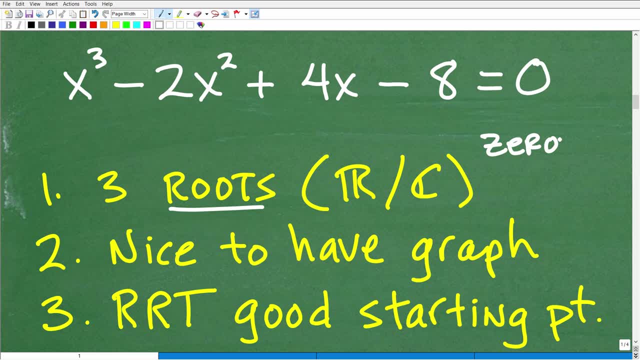 And you might hear another word: zeros, roots and solutions. Basically, you're trying to solve this thing. You're trying to find the solutions to the polynomial equation, But all these words are very common: Roots, zeros and solutions. All right. 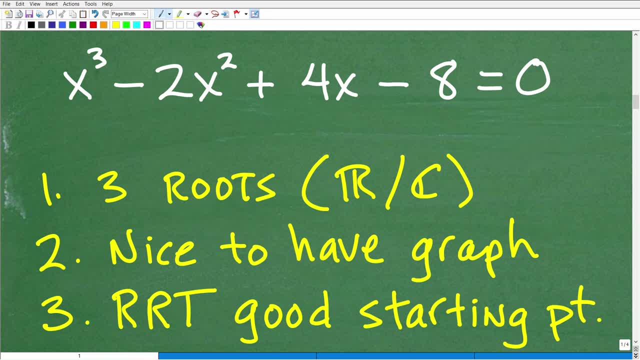 Again, they're pretty much synonymous And again, the first thing we want to do is like: OK, we know we are looking for three roots, right, Three solutions because of the fundamental theorem of algebra. I just don't know if they're going to be real numbers or complex numbers, or imaginary numbers. 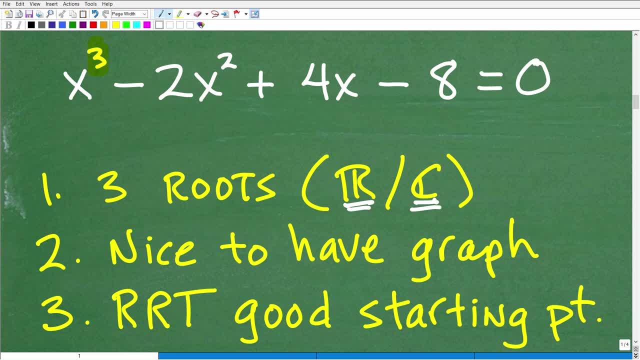 You just don't know that right now. Do you know, going into this problem, that you will find three solutions? So that's the first thing. Now the second thing is: it's definitely nice to have the graph. OK, if you have the graph, if you're able to. let's suppose your teacher says yes, you can use a graphing calculator. 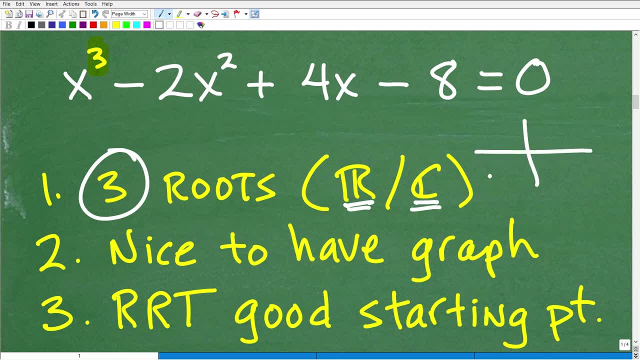 You definitely want to take a look at the graph because the graph can give you hints. Anywhere the graph crosses the X axis are actually locations of real number solutions, real roots. OK, So the graph is like super valuable, So you definitely need to know how to use a graphing calculator. 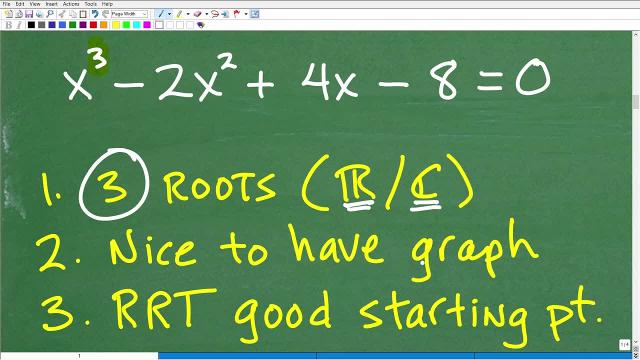 But we're not going to use this, But it's not. It is definitely nice to have the graph and to graph these things, But this is part of kind of like forming a game plan here. So the graph could definitely give us huge clues on where these are, where and what type of solutions we have. 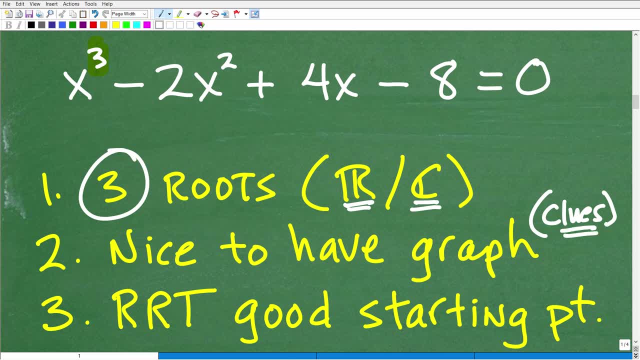 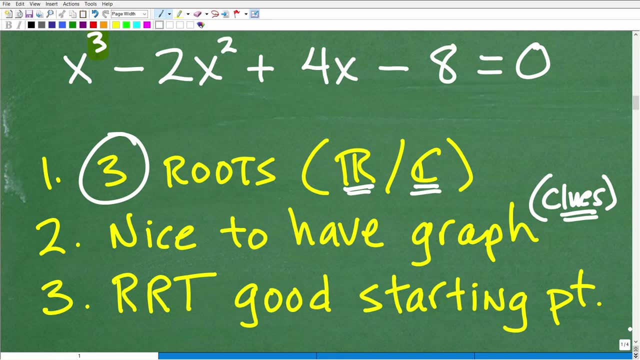 OK, But again we're not going to use it in this particular problem. But the last thing we're going to be talking about- And this is kind of again structuring our game plan to kind of tackle this problem- is using the rational root theorem. 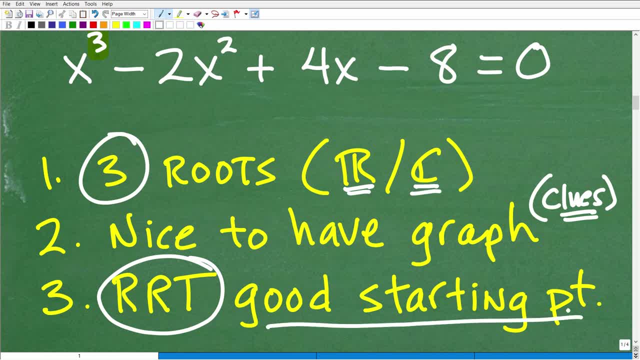 And this is a great starting point. So when you don't have any other kind of things that are obvious to do, you know most of your teachers or textbooks are going to say: just get right into the rational root theorem, OK. So what does that mean? 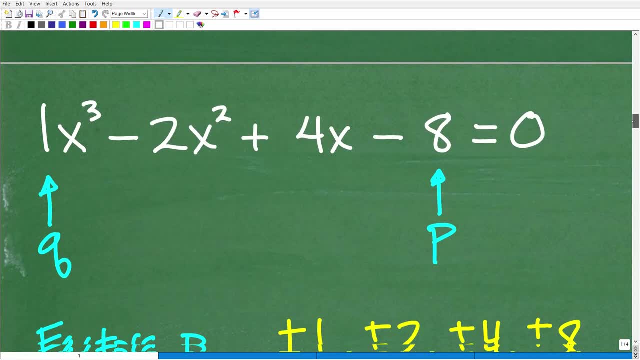 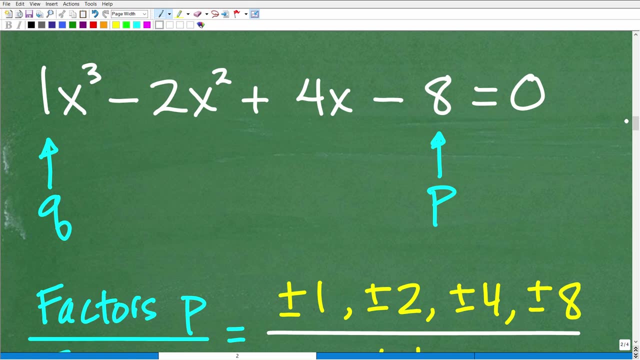 Let's go and talk about that right now. All right, So the rational root theorem. Again, I'm kind of covering a lot of ground here, that you need to look at this more thoroughly. But effectively, this polynomial equation- Right, We know that it has three roots. 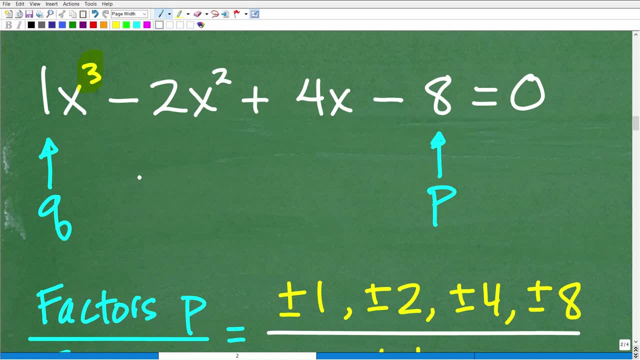 OK, Now what type of roots does it have? Again, we don't know if it's a real number of roots, They're complex or imaginary roots. But here's the thing: They may or may not They, this polynomial equation may. 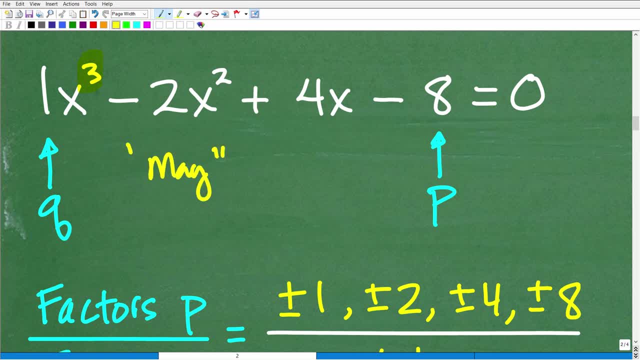 And I'm going to really emphasize this word- may have, OK, Some rational roots, Rational roots. So what are rational roots? What are rational numbers? Rational numbers are basically numbers that are fractions that are made from integers, Things like one, half, three, fifths, six. 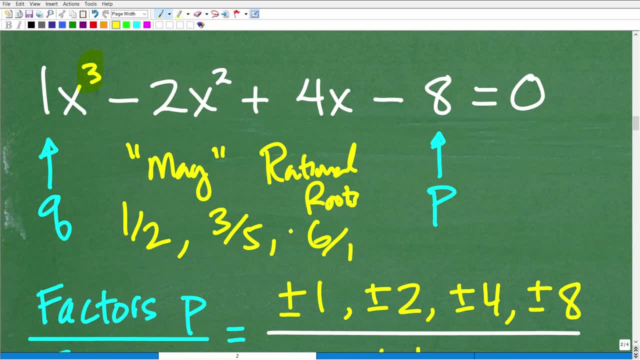 Right, Because you can write six as six over one. So these are rational numbers. Hopefully you remember that. OK, But these are examples of rational numbers. So the rational root theorem is basically: it's a wonderful theorem And it says: hey look, this thing may have rational roots. 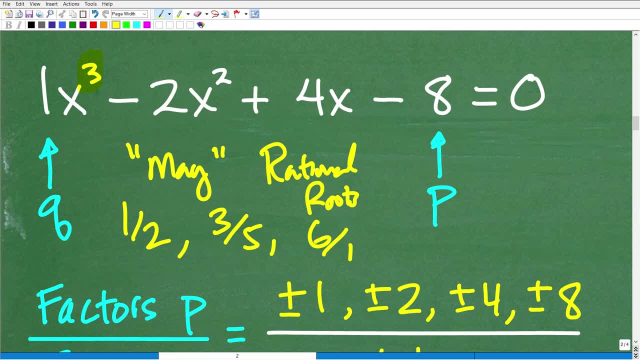 It may not OK, But if it does have rational roots, we can kind of make a list And we're going to construct a list right now, And if this thing does have rational roots, it'll be amongst this possible list of numbers. 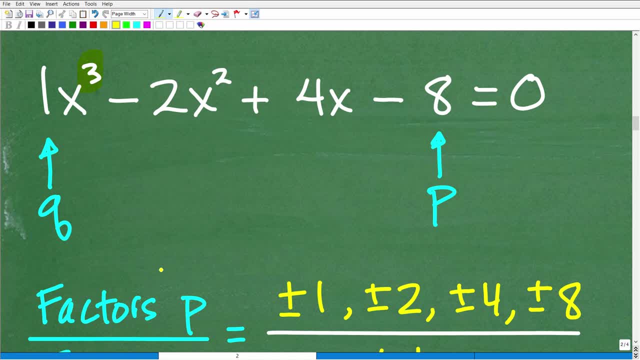 So here's how this thing works, OK. So first of all, notice that we have a number, OK. Well, notice that our polynomial equation is written in standard form: highest to lowest power. OK, And our first leading coefficient here is going to be q. 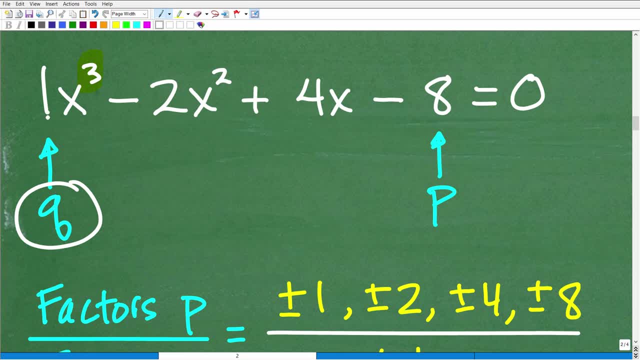 OK, So q, this variable q, we're going to assign as the value of this leading coefficient, which of course is one, And then p is going to be our constant value, which of course here is eight. All right, 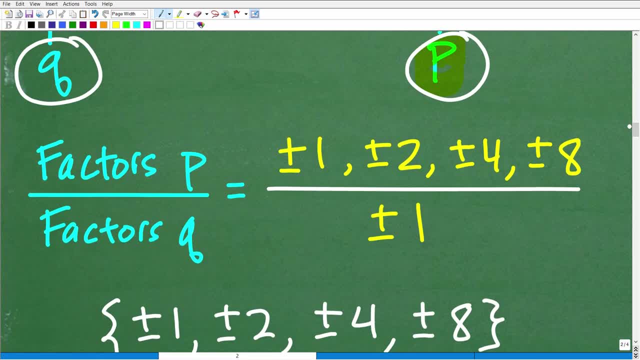 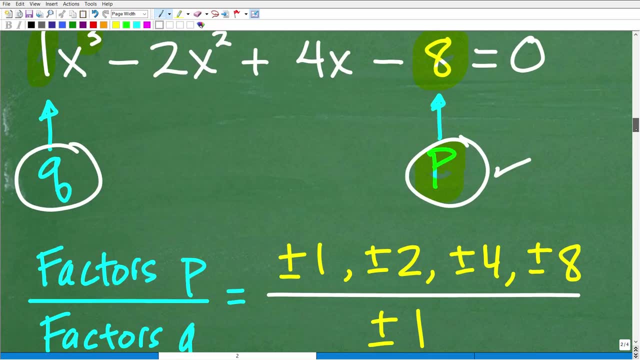 So the rational root theorem says: OK, take the factors of p, Which of course is eight in our problem- OK, You can see that right there- And the factors of q. So we're going to construct all the factors of p. 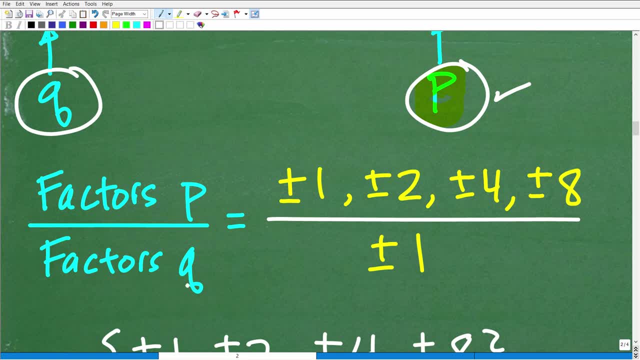 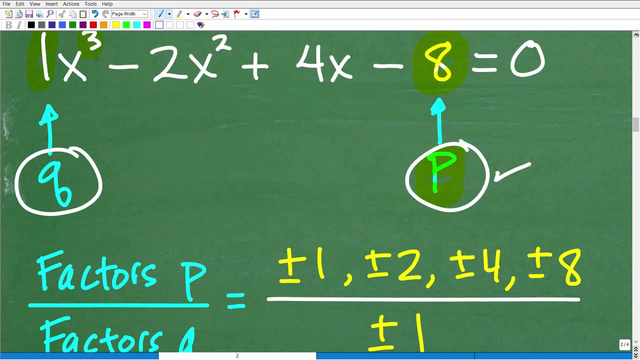 And we're going to divide that over all the factors of q And then, once we kind of simplify this, we will have a list of all the possible rational roots. So the way you do this is the following: OK, We're going to take eight right here. 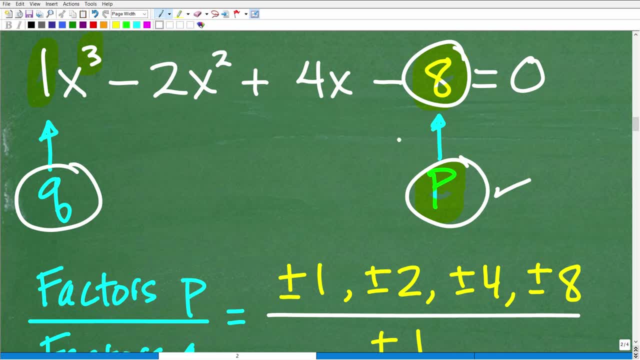 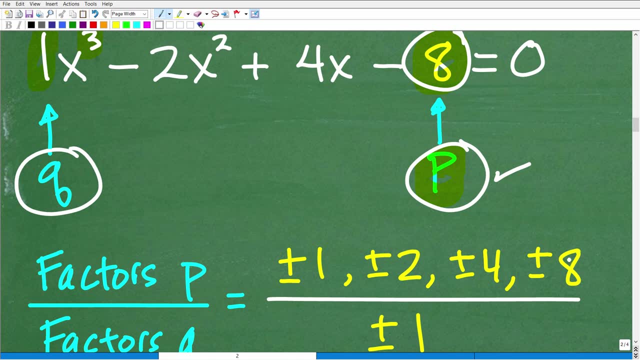 And we're going to start with all the factors of eight. OK, So what are factors of eight? Well, one, OK, is a factor of eight, Two is a factor of eight, Four is a factor of eight, And eight is a factor of eight. 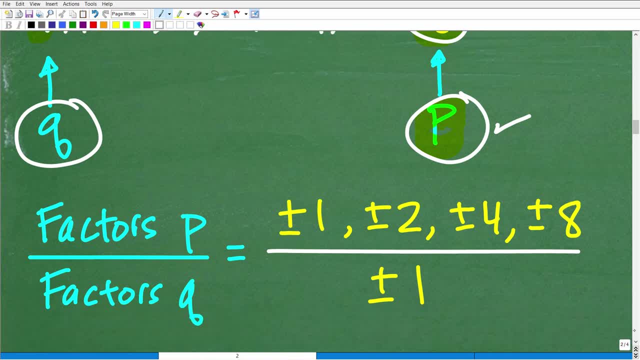 Now, if you've never seen the rational root theorem, OK, I'm just telling you right now. you have to put plus and minus into all of these. OK, Because positive two times positive four is going to be eight. Negative two times negative four is also positive eight. 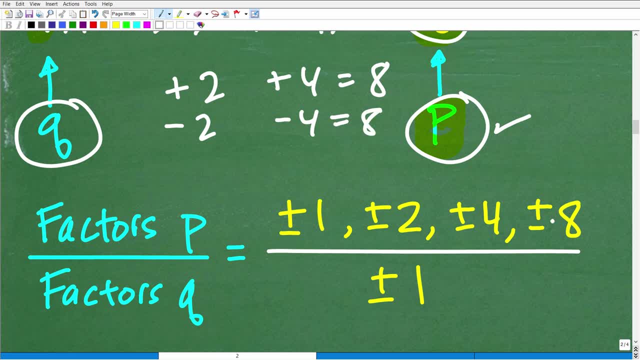 So just get in the habit of putting plus or minuses for all your factors. That is our numerator. Now again, if you're confused with this just basically means that you need a lot of follow on instruction. This is a lot in and of itself. 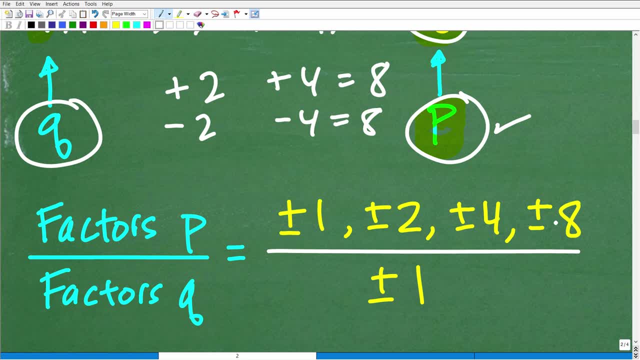 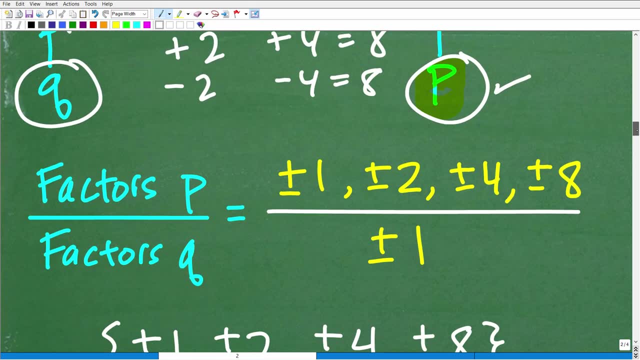 So again, I'll just direct you to those courses I talked about. OK, So what is q? Again, q is just one. So the factors of one- that's pretty easy- is plus or minus one. OK, So we can see that right there. 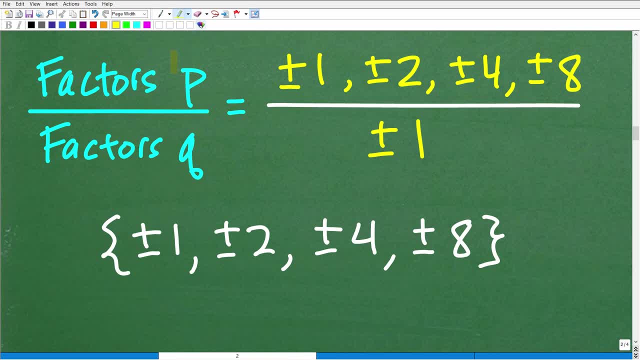 So now let's go ahead and clean this list up, And here's how we're going to do this. We'll just take we got only one number, one factor, One factor down here in our denominator, So plus or minus one divided by plus or minus one. 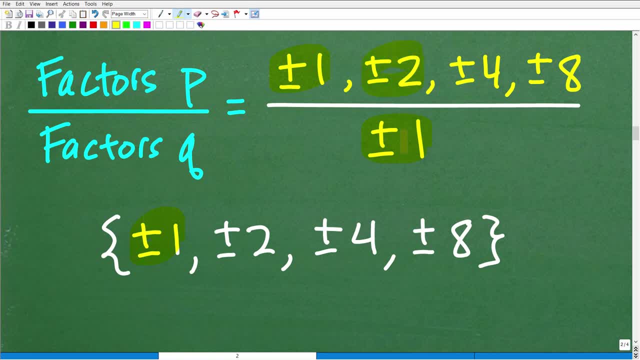 Easy, That's: plus or minus one, Plus or minus two, divided by plus or minus one, plus or minus two, Plus or minus four. divided by plus or minus one will give us a plus or minus four, And then plus or minus eight. divided by plus or minus one is plus or minus eight. 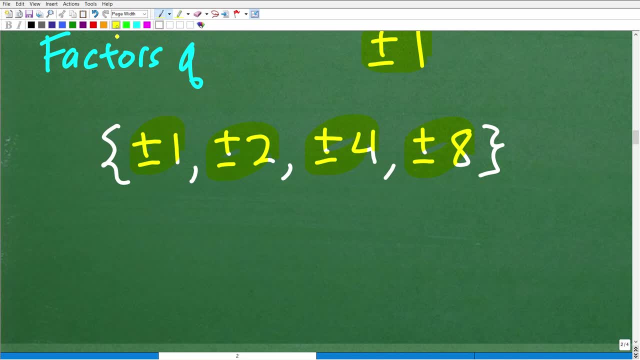 So what does that mean? Well, let me write this all out the long way. So one negative one, two negative two, four negative four and eight negative eight. if this polynomial has rational roots, okay, it will be amongst this list, okay, and so this is obvious. this is great, because we're basically saying is like: hey, look, one of 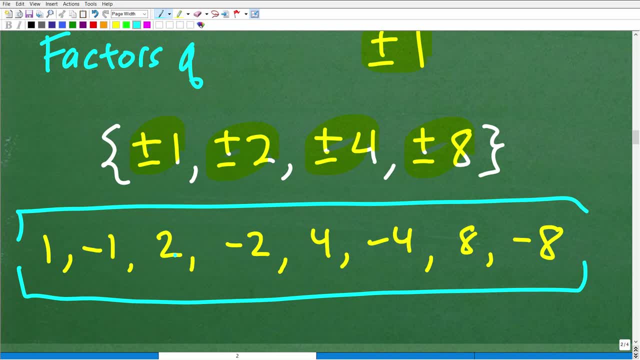 these right here might be one or three of these, might be our three solutions now, because you work out that none of these are solutions as well. okay, so we just don't know. so what do we do here? well, now we have to kind of start to try these solutions. this is the strategy that you need. 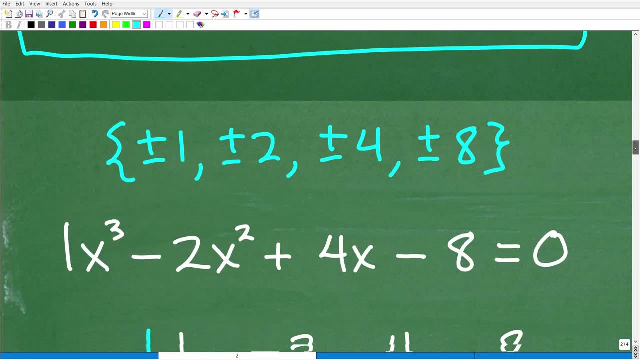 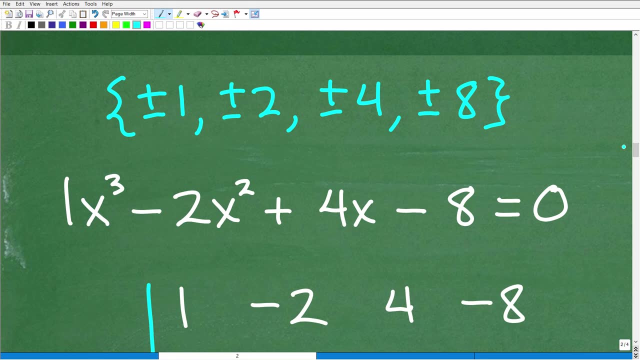 to take. all right. so let's take our list of possible rational roots- and here is the list, and we're going to go ahead and start checking these solutions to see- or check these possible solutions, excuse me- to see if we can find any solutions. okay, so how do we do this? well, this: 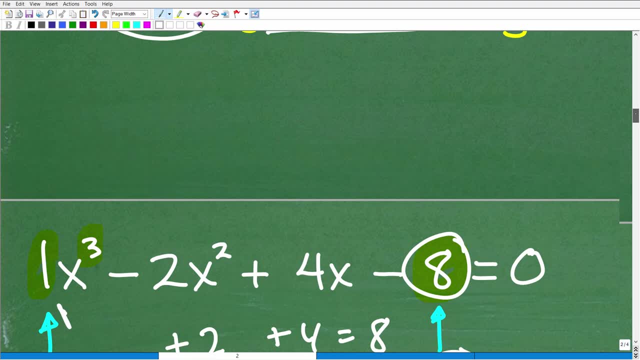 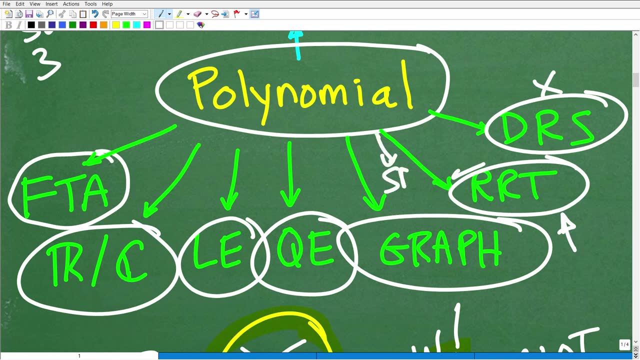 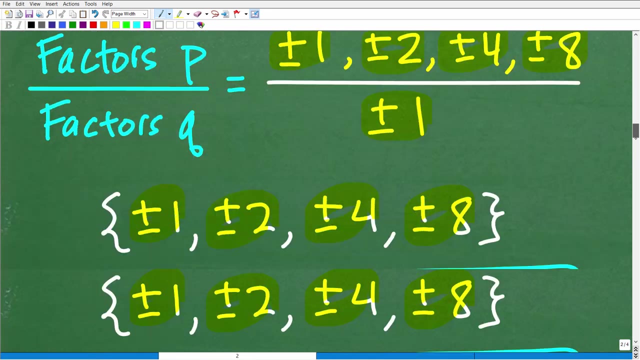 brings us to the next thing and, by the way, maybe i could put this way up on our lovely list up here. let me go way up here. i told you i left a lot of things out over here you could put in: synthetic division, long division. so again, wow, that's a lot. yes, i know it is a lot, but nothing that you cannot handle. all right, let's. 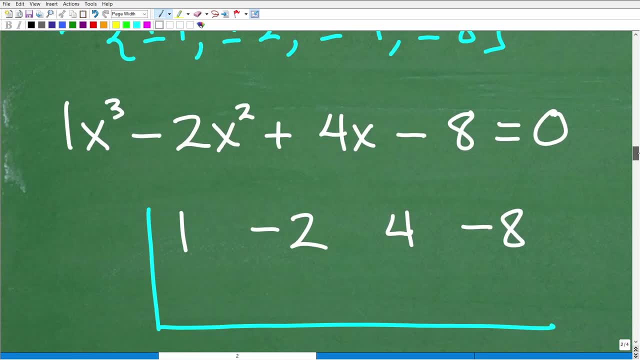 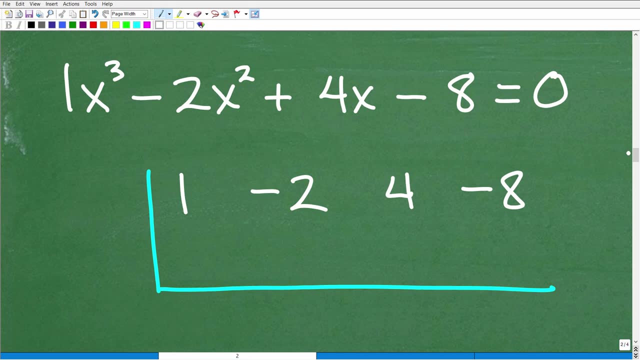 get back to the problem here, okay, so now let's start checking um, uh, these, uh, possible rational roots. so the way you're going to do this is use something called synthetic division. and the way synthetic division works is: notice again, we have our polynomial in standard form. we're going to take the coefficients, okay, so we have one negative two, four and negative eight. 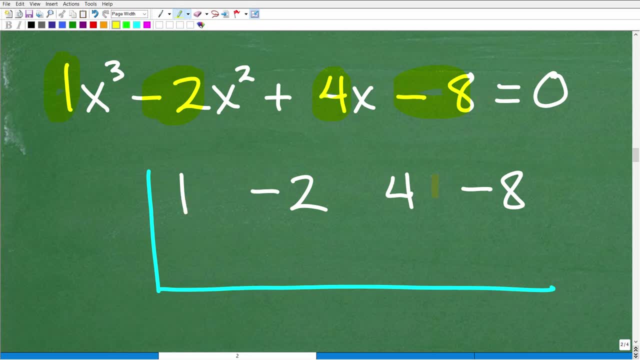 okay, so here's all this, and you can see, we're just going to write them in this order and they're going to make a little bracket like an l bracket, just like that. okay, so this is. there's another kind of format that you can use, but this is the most common. all right, so that's step one. so let's. 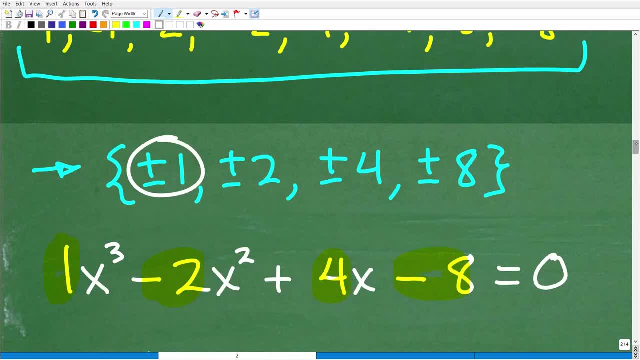 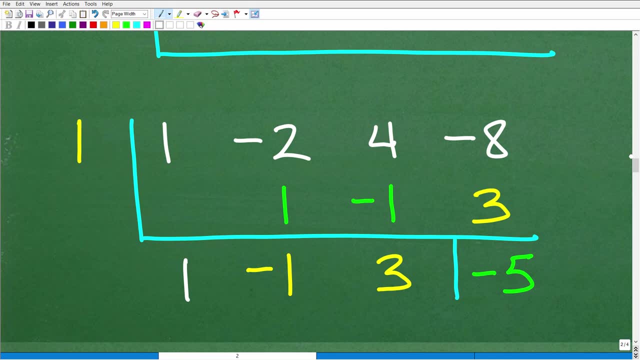 go ahead and check, uh, one of the roots right now. how about we check positive one? so here is the procedure to use for synthetic division. so here you can see. i already did the work, so i'm going to explain this to you. i know i'm covering a lot of ground quickly. 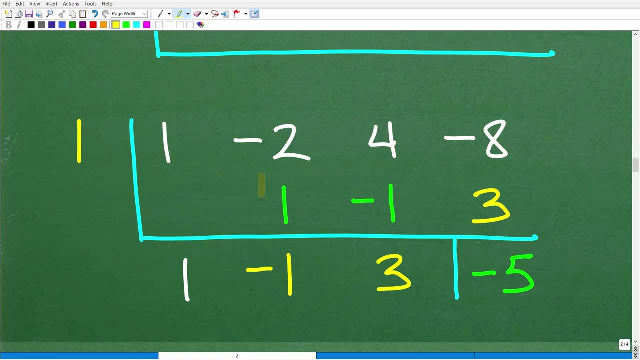 so just make a note of what you don't understand. but here's how synthetic division works. okay, so we always start with the very, very first number one. so we're going to drop that down right here. okay, so you see that one gets dropped down to one. now the next thing i'm going to do is you're going. 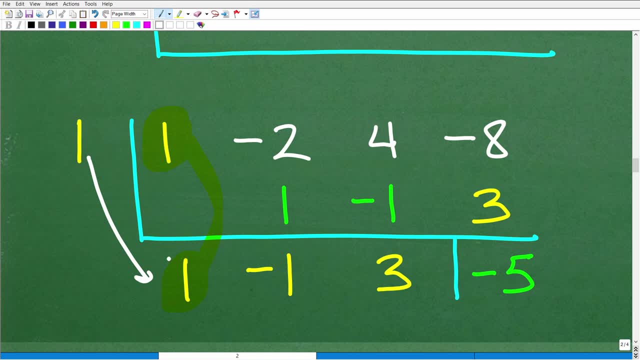 to take that one and multiply. you're going to take whatever number this is and multiply by that number. so one times one is what it is one. we put the answer right here. then we add down: so negative two plus one is what negative one. all right, so hopefully you're following me on that. 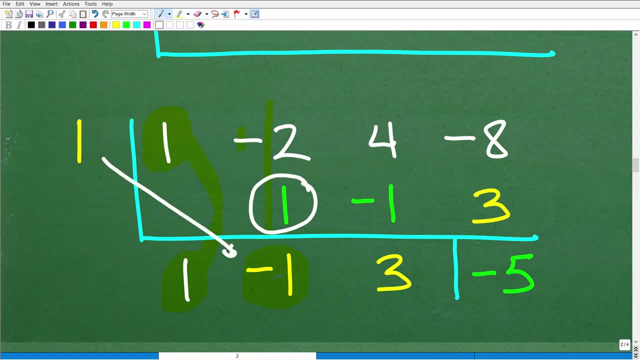 and then we're just going to repeat the procedure. okay, so one times negative one is what that is a negative one, and then we add down four plus negative one is positive three. okay, now we'll just continue on with the procedure here. so one times a positive three, of course, is positive three, and then we add down, we get. 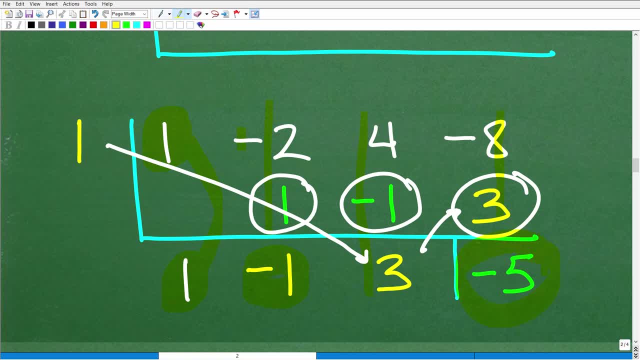 negative eight plus three is negative five. so this is a synthetic division and this kind of gets into another concept here called the remainder theorem, right? so this is a whole. again a lot going on here. but here's the deal, right, if one okay was in fact a solution to this polynomial. 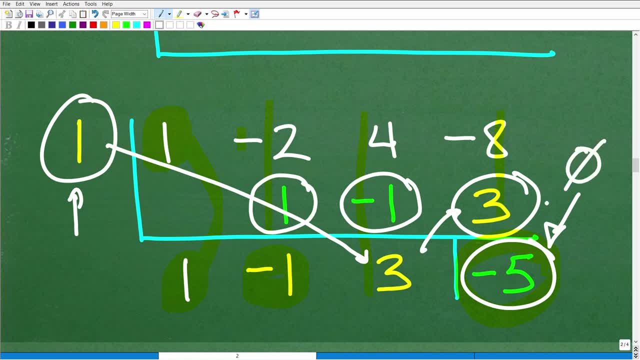 equation. this remainder would end up being the remainder of the equation. so we're going to isolate zero. okay, and obviously it is not. so what's this tell us about? one is one is not a solution, so we can throw that out. and so what do we do? well, listen, we only check positive one. 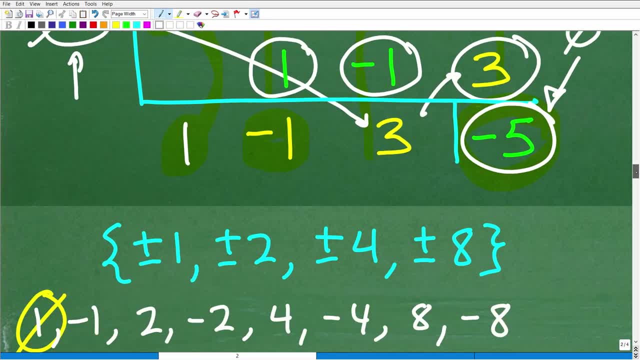 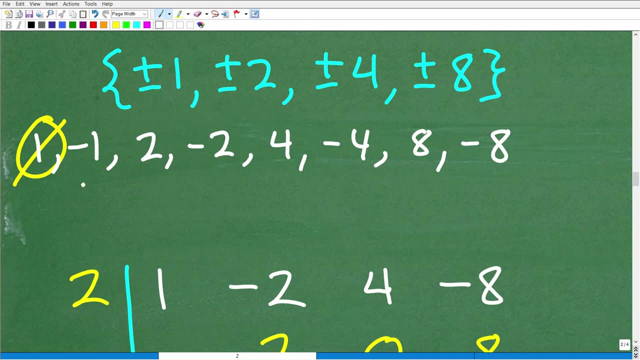 we need to continue to check all of these numbers and you're like boy, that's a lot of work. yes, it is, but you know, have fun with it. okay. so we tried one. it doesn't work now, just for interest of time. uh, negative one does not work, okay, so let's suppose. 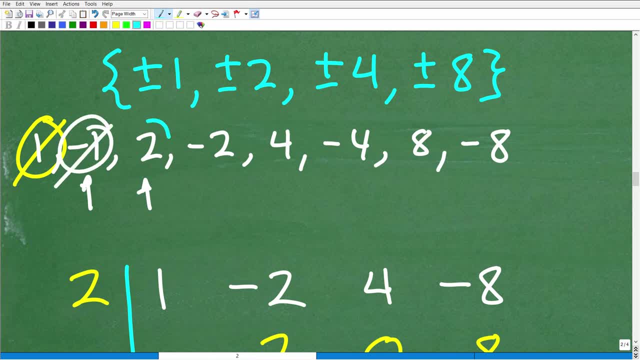 on to our lovely list. wow, that didn't work either. and then we went on to two. so remember, at the beginning of the video i gave you the answer and two was a real number solution. so we know that this is a solution, but let's suppose we didn't know that we're going through our lovely list. 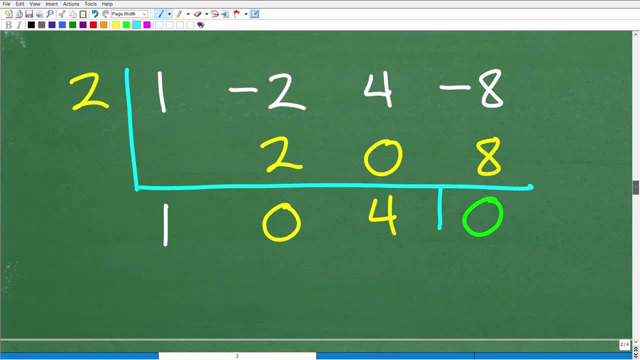 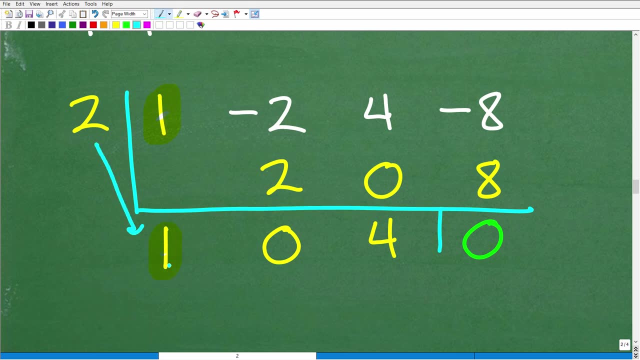 and now we run into two. so we're going to try two. so let's go ahead and do that right now. so again, we're going to start with this one, we're going to drop it down and then we're going to go two times. one is uh, two. we put our answer here: add down negative two plus a positive two is zero. 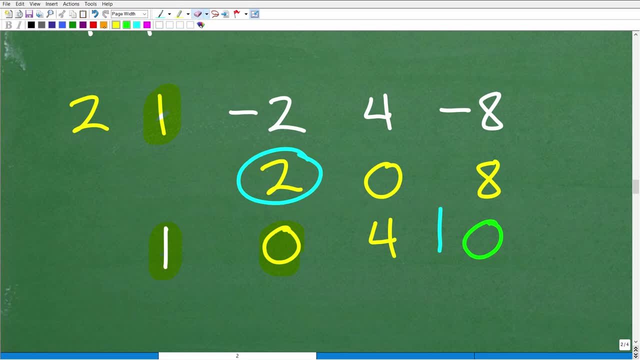 okay, so we continue on. uh, whoops, whoa, i didn't mean to do that. uh, so then we have two times zero, of course. is what zero? okay, add down four times zero, or sorry, four plus zero is four, and then we're going to just do this again. two times four is what? 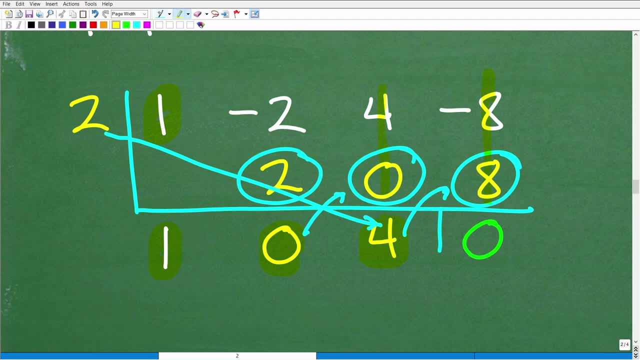 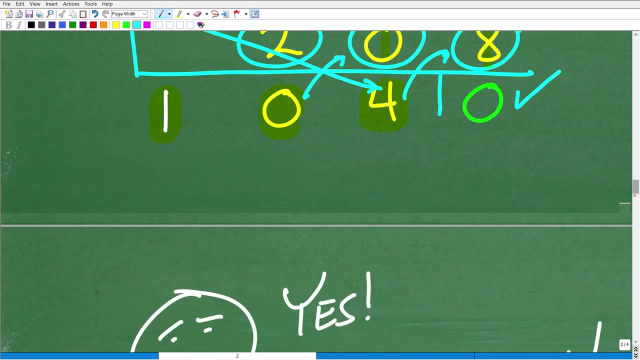 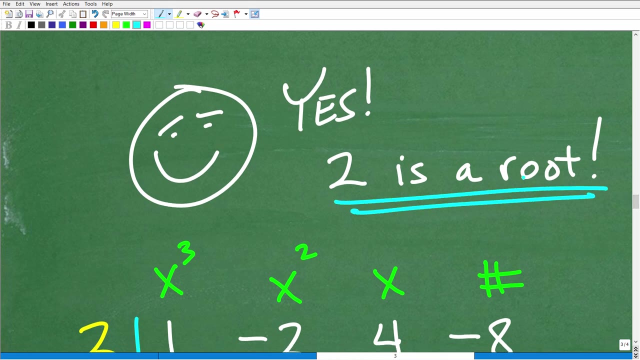 eight. and finally, when we add right here, we're like, oh, this is super awesome. negative eight plus a positive eight is zero, and that means what that means: two is a solution and we can celebrate: yes, we got one. two is a root. okay. now, this is very awesome. okay, and i'll tell you why. because 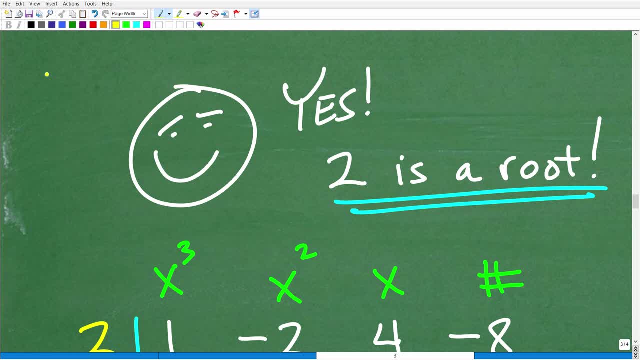 in algebra, if you recall, you got really good at solving quadratic equations, which are second degree polynomials. so you know you have techniques that guarantee you do find the solution to quadratic equations, remember. uh, if you use any technique and it doesn't work, you could always go to the quadratic. 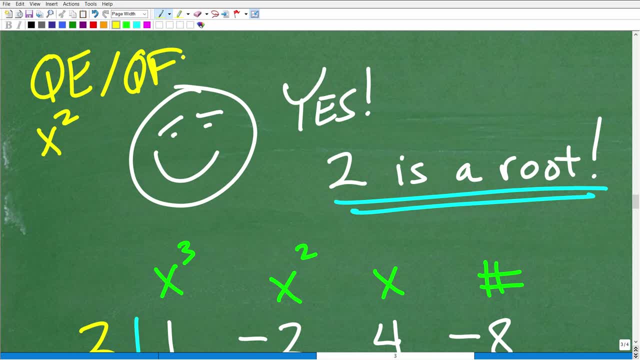 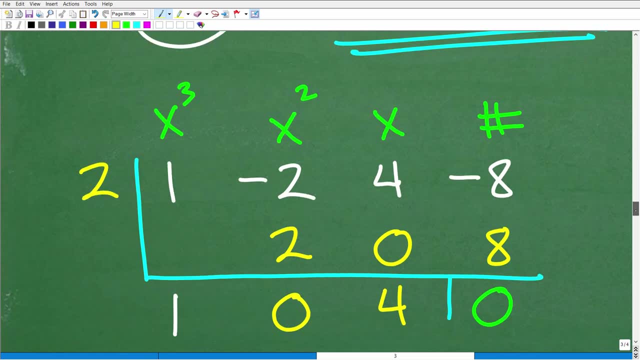 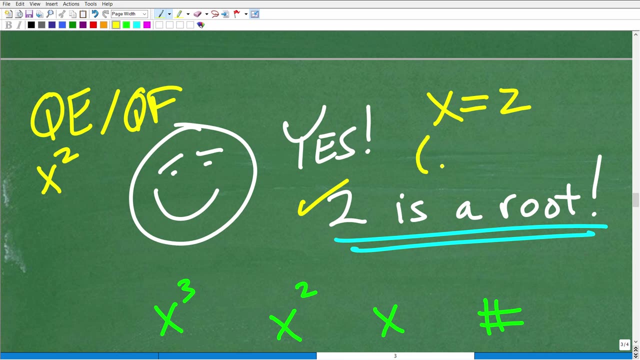 formula and solve any quadratic equation. all right. so this is a really good find for us. a two is a root, so what does that mean? okay, well, effectively means that x equals two, one of the roots equals two, and that can come from here. there's another topic: the linear factor x. 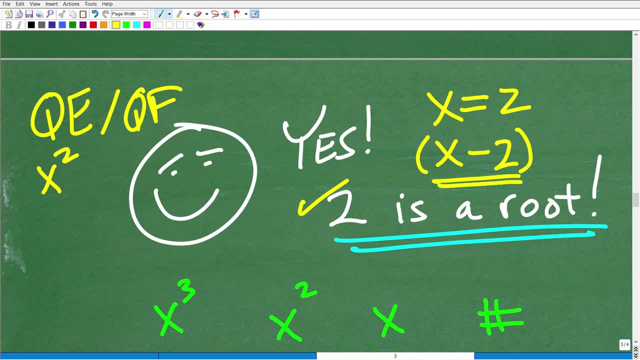 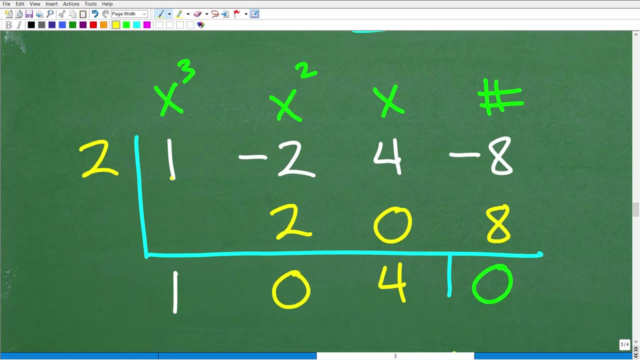 minus two. okay, i'll explain what i'm talking about here in a second. but more importantly, we have to go back to our synthetic division and remember here are the coefficients to our polynomial. remember we have 1, negative 2,, 4, negative 8. 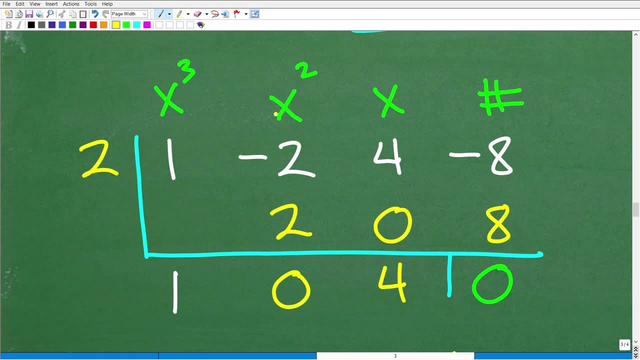 well, look at the columns here. 1 was the coefficient of x cubed right negative. 2 was the coefficient of x squared uh. four was the coefficient of x negative. eight was the coefficient or just the constant number 18, When you do synthetic division, whatever the answer is down here, the degrees go down by 1, okay. 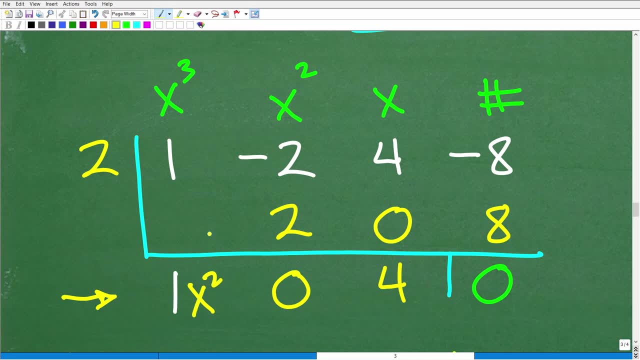 In other words, instead of x cubed, this is now x squared. okay, So this goes down by 1.. Instead of x squared, our answer here is x, so 0x. And then, instead of 4 to the first, this is now our constant. 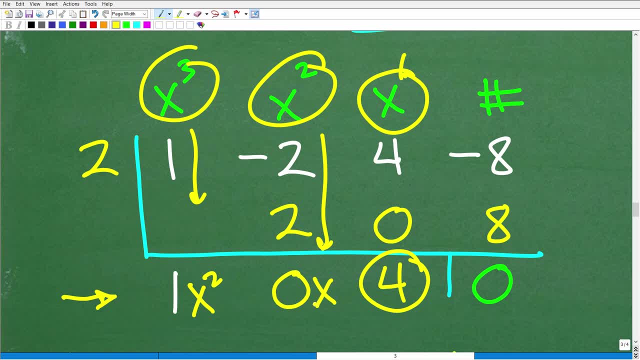 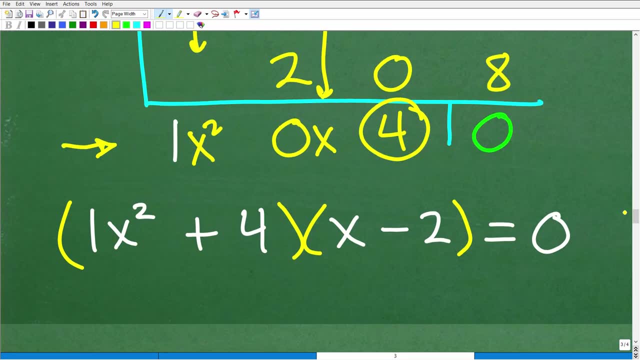 So really, what we have here is x squared plus 0x, which is 0, or x squared plus 4, okay, So that's what is the result of doing synthetic division by 2, okay, We're talking about polynomial division here. 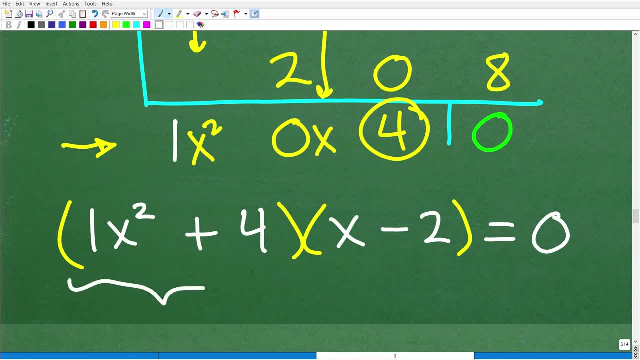 So what you need to be able to identify is that we're talking about the linear factor x squared plus 4, okay, We already have x minus 2 equal, because all this right here, if we had this and we set this equal to 0,. 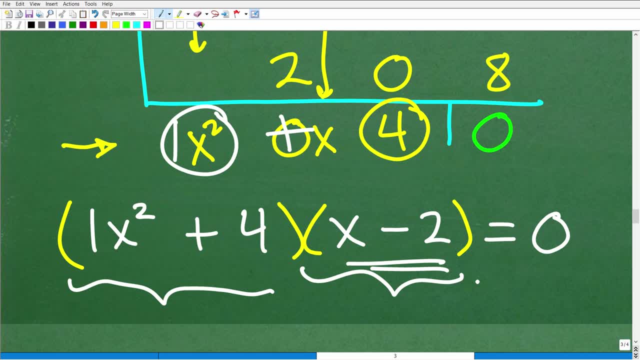 we would set this factor equal to 0 and solve. We would get x is equal to 2, which we know is a solution All right. So if you are with me so far, then that is outstanding. If you're completely lost, do not panic. 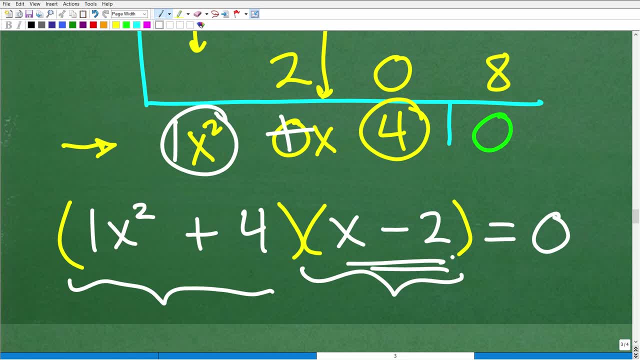 Just be like: okay, I got to get more instruction on this and that's what you need. This is not going to come, you know. you can't just, you know, put a little bit of work in here and expect to master all this stuff. 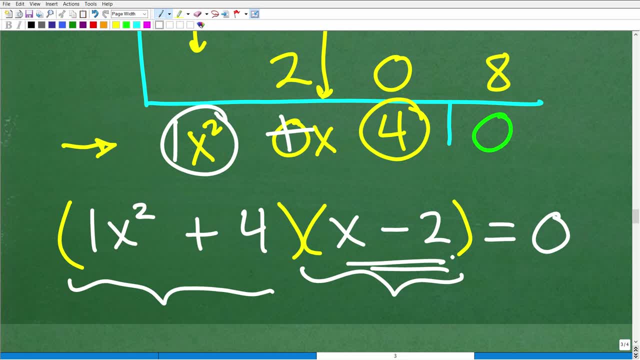 You really have to work hard to do this. You can do it, It's just, you know, all based upon your level of commitment. Okay, So here we already have the solution to this. This is: x is equal to 2.. 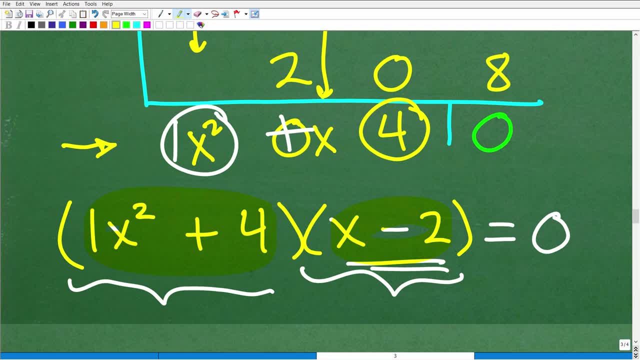 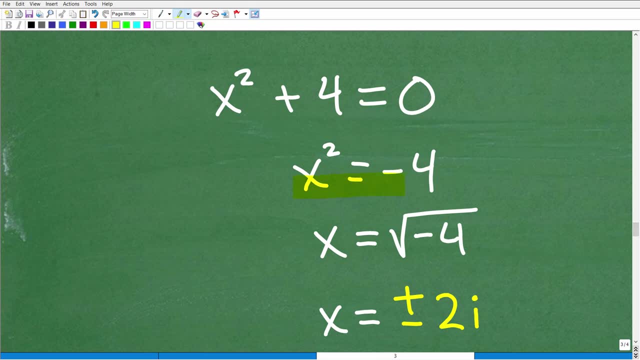 That's our Positive root. So let's go ahead and now deal with x squared plus 4 and set that equal to 0.. Okay, So x plus 4 equal to 0.. Going to move the 4 to the other side. 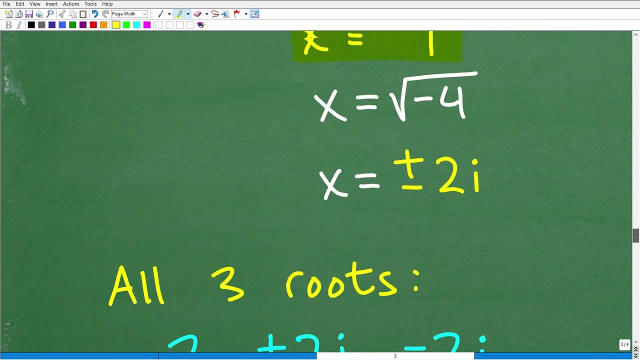 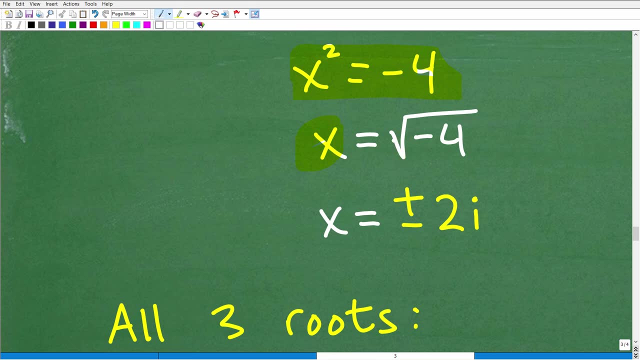 We got x squared is equal to negative 4. And you can see what's going to go on here. When I take the square root of both sides right to solve for x, I'm going to have x is equal to. Actually I should put in a little positive or negative right there. 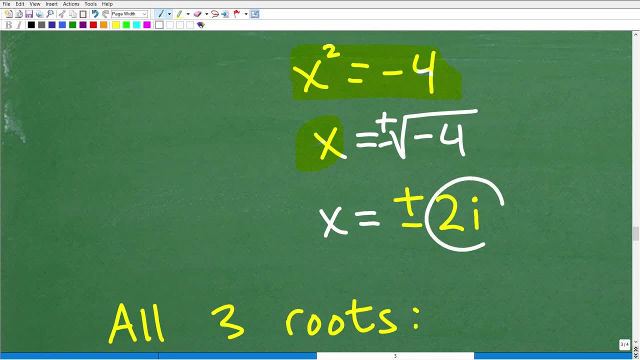 The square root of negative 4 and the square root of negative 4,, of course, is 2i. So we have that positive negative 2i. So of course we're talking about imaginary and complex numbers, right? So just to be clear on complex, a complex number is written in the form of a plus b i. 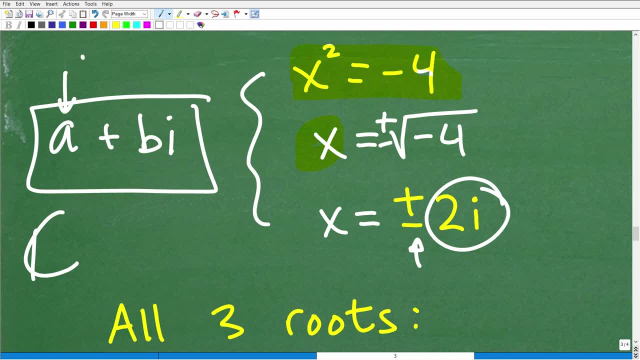 This is a complex number. Okay, This component here is the real number component And this component here is the imaginary number component. So you know again, you don't want to be. you want to use these descriptions correctly when you're talking about the type of numbers and type of solutions that you're dealing with. 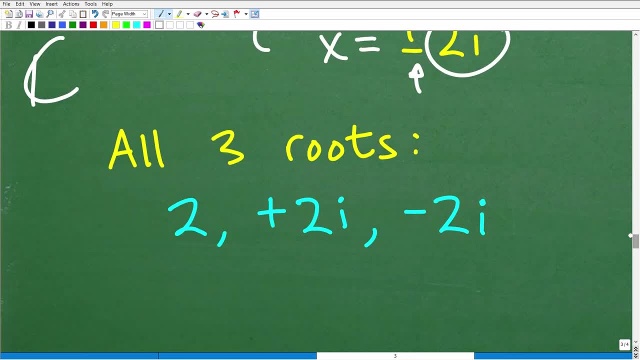 Okay. So what does that mean? Well, it means we've found all three roots. Okay, We've found two. Two is a real number solution. And how do we find two? Well, we need to start someplace. We use the rational root theorem. 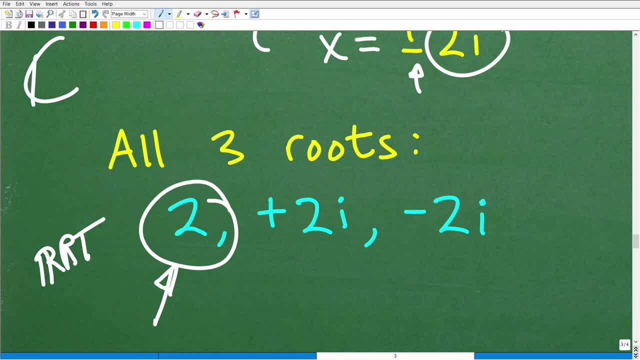 And we tested that, And we were lucky enough for this particular problem to have a rational root, And then what was left was a quadratic equation, Okay, With imaginary solutions, And we have our positive 2i and negative 2i As the last two remaining roots. 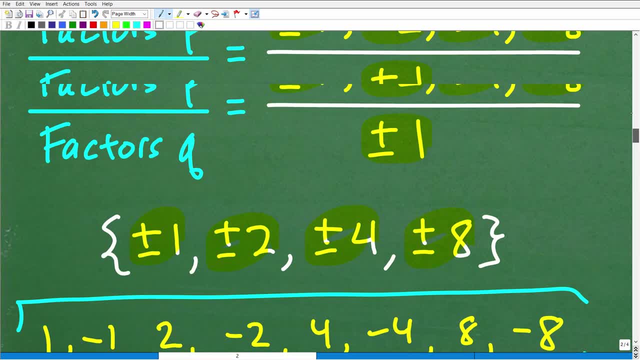 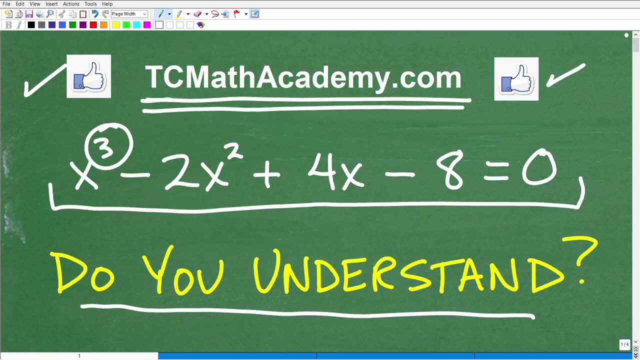 Okay, So I know I covered a lot of information in this video, But I would say that this is pretty. this is like an average level problem at this at. you know this level of mathematics. So if you're like, what do you talk about?